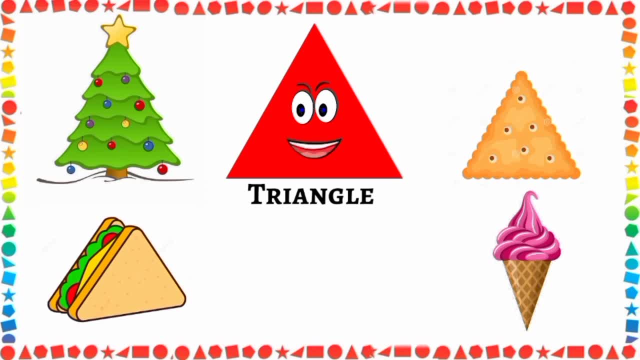 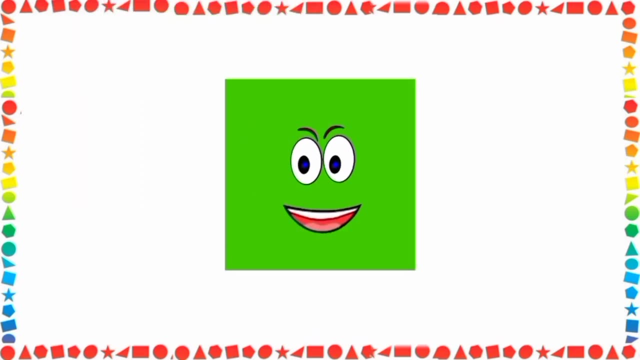 You can enjoy me as an ice cream cone. You can eat me as a pizza slice. All three sides make me a triangle. All these objects can be seen in the shape of a triangle. Hi, I am a square. I have four equal sides. 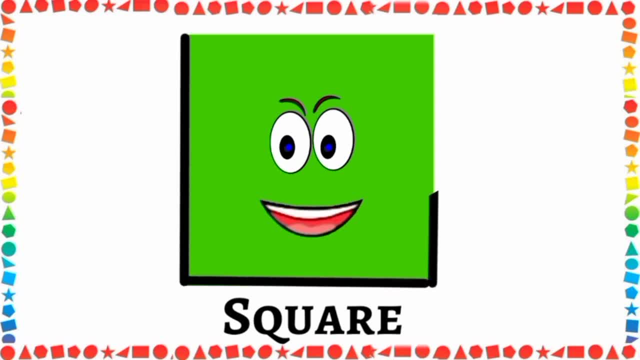 One, two, three and four. I have four equal sides and four corners too. One, two, three and four. My four sides and four corners make me a triangle. My four corners make me a square. You can find me anywhere around your surroundings. 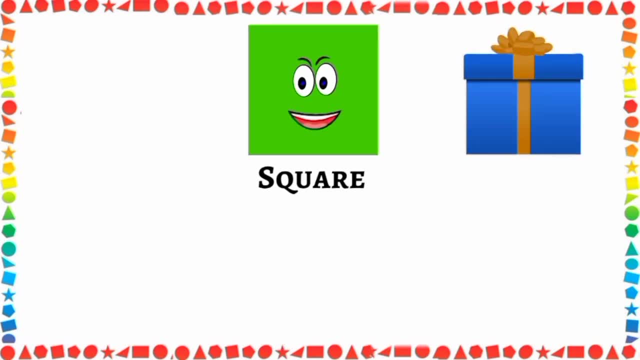 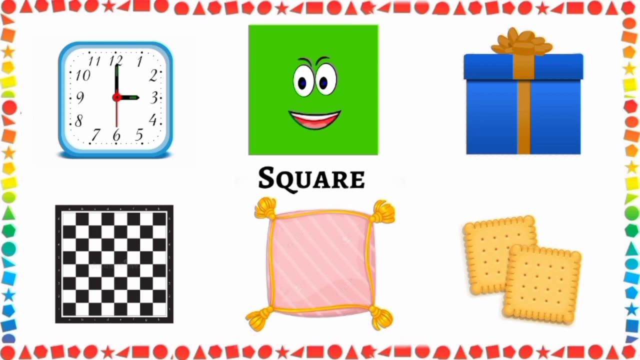 For example, you can wrap me as a gift box, You can watch me as a wall clock, You can play on me as a chess board, You can eat me as a cookie, You can rest on me as a pillow. All these objects can be seen in the shape of a square. 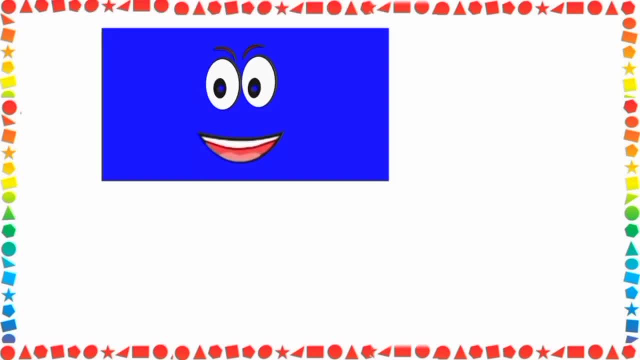 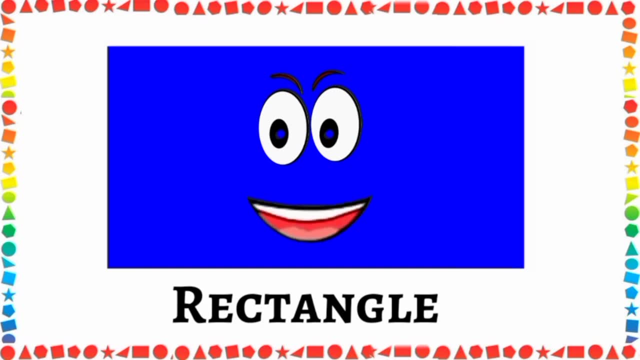 Remember to subscribe to my channel. Thank you, Hi. I am a rectangle. I have four sides. My opposite sides are equal: One, two, three and four. I have four sides and four corners too: One, two, three and four. 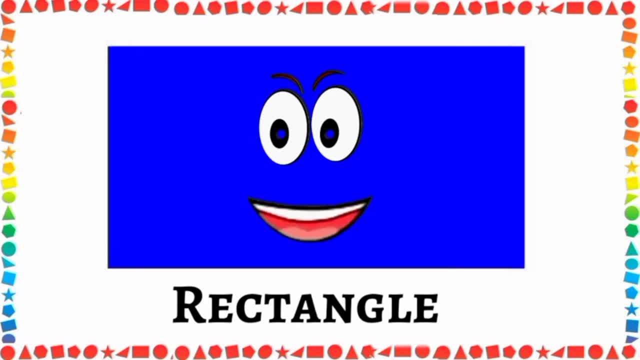 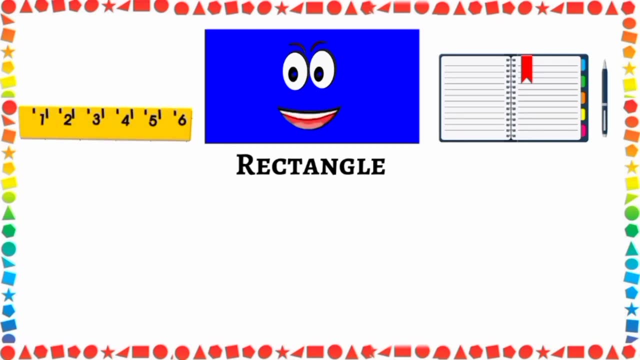 My opposite side is equal. Opposite equal sides and four corners make me a rectangle. You can find me anywhere around your surroundings. For example, you can write on me as a notebook. You can use me to measure things as a ruler. You can use me as a green board. 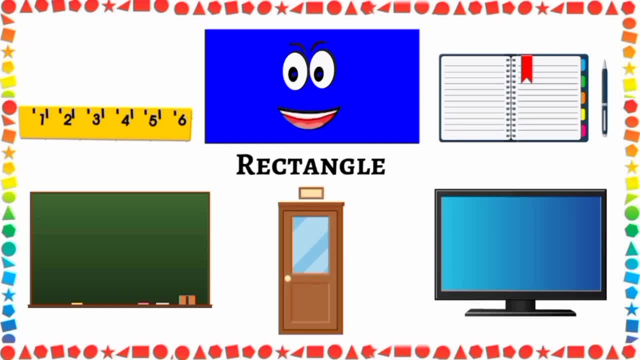 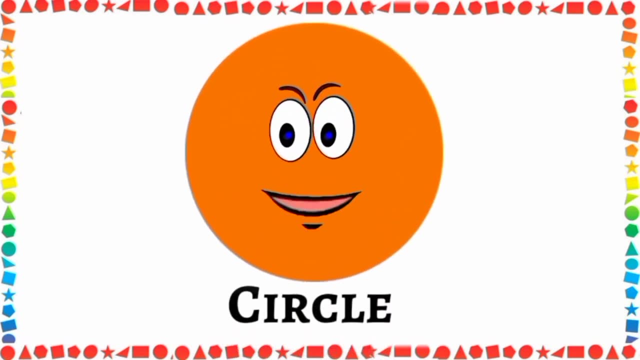 You can watch me as a television, You can open me as a door. All these objects can be found in a shape of a rectangle. Hi, I am a circle, I am round in shape and I am made up of only one curved line. 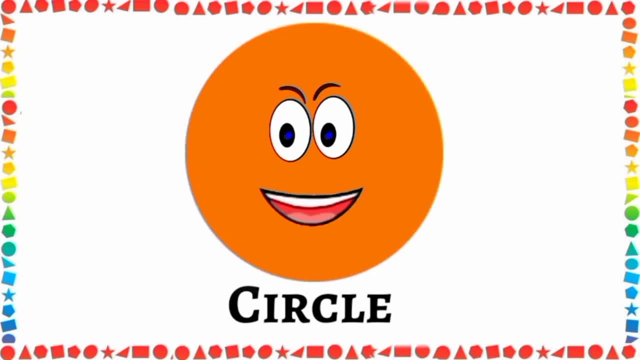 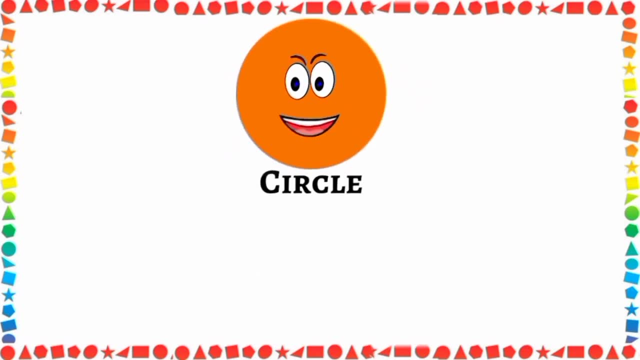 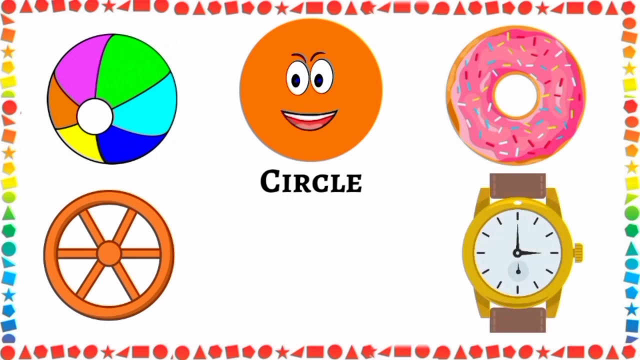 I have no sides and no corners. You can find me in many objects present in your surroundings. For example, you can eat me as a doughnut, You can play me as a ball, You can roll me as a wheel, You can tie me as a watch. 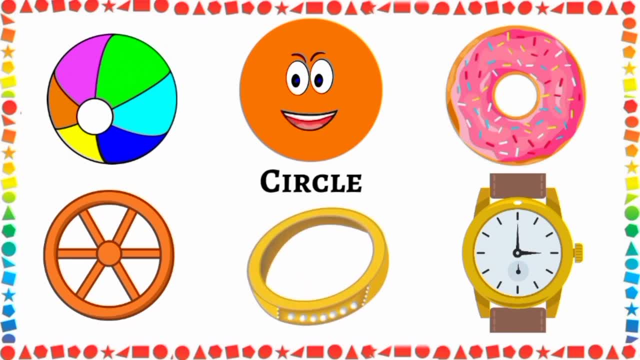 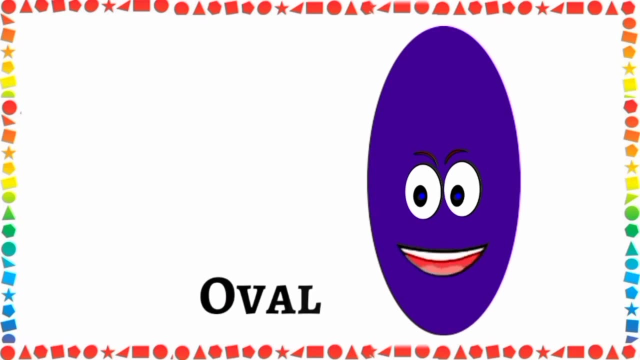 You can wear me as a bracelet. All these objects can be seen in a shape of a circle. Hi, I am an oval. I have no sides and no corners. I am made up of one curved line. You can find me in many things around your surroundings. 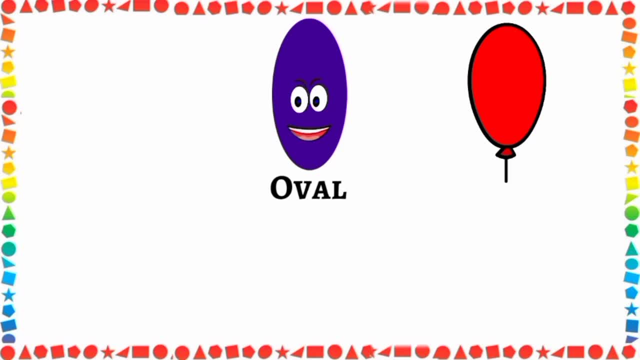 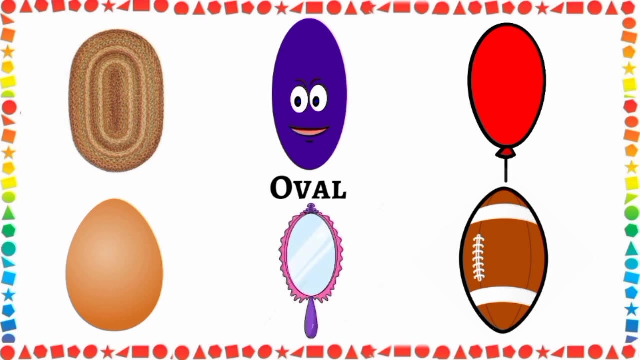 For example, you can blow me as a balloon, You can use me as a doormat, You can eat me as an egg, You can play with me as an American football. You can use me as a mirror. All these objects can be seen in a shape of an oval. 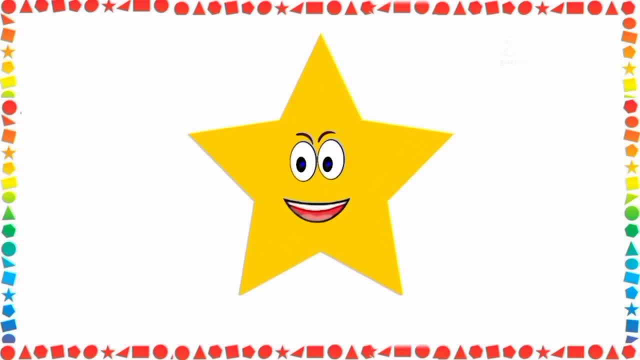 Hi, I am a star. Let's move and count my sides: One, two, three, four, five, six, seven, eight, nine and ten. I am a shape with ten sides and five corners: One, two, three, four and five. 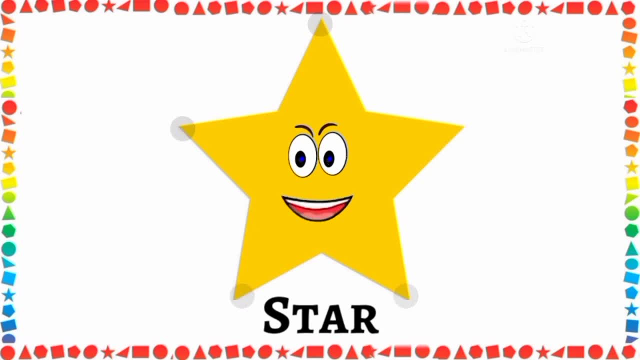 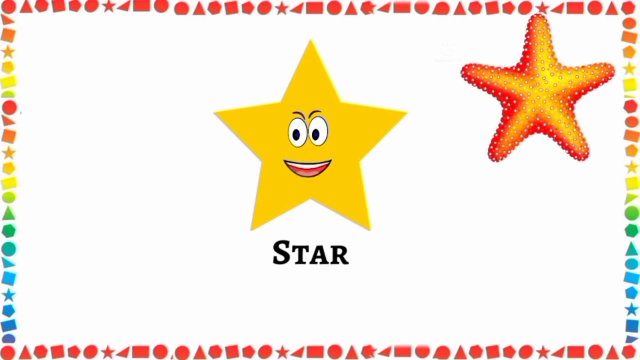 I have ten sides and five corners: One, two, three, four and five. I am a shape with ten sides and five corners- corners. You can see me in many things around your surroundings. For example, you can see me as a starfish. You can use me as a star balloon. You can see me in a magic wand. You 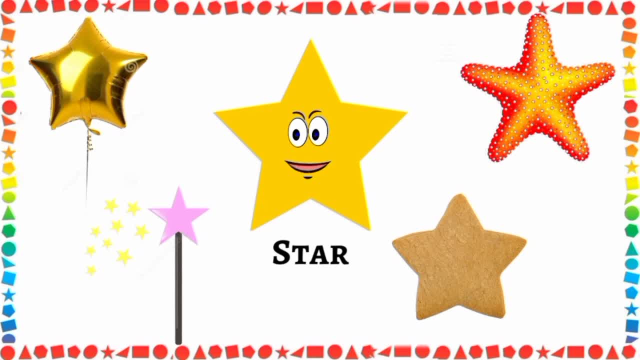 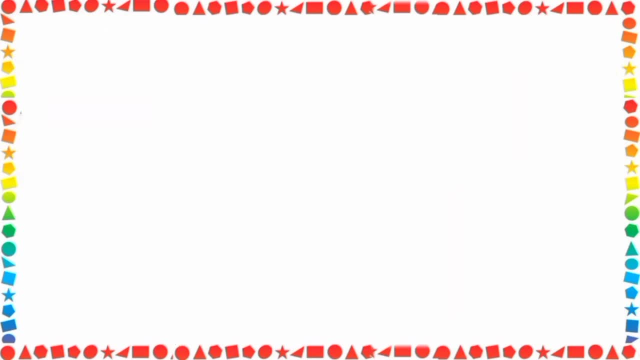 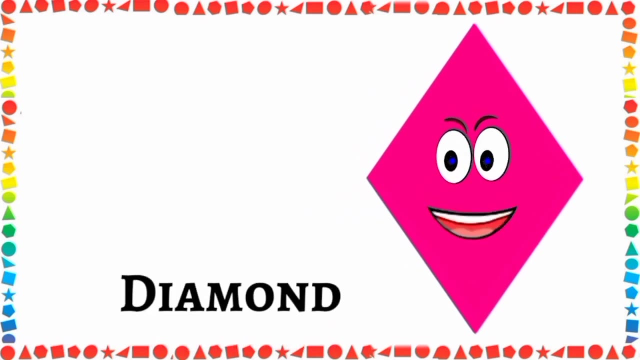 can eat me as a star cookie. All these objects can be seen in a shape of a star. Hi, I am a diamond. I have four sides: one, two, three and four. I am made of four sides and four corners. 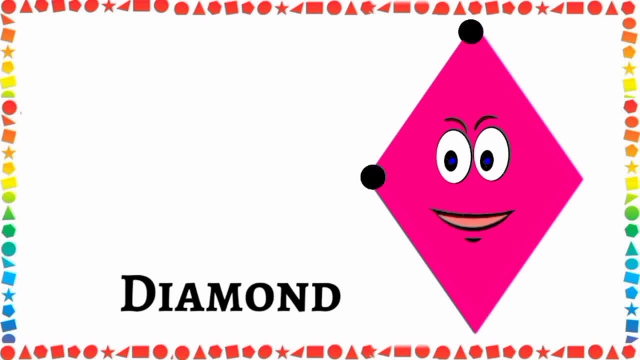 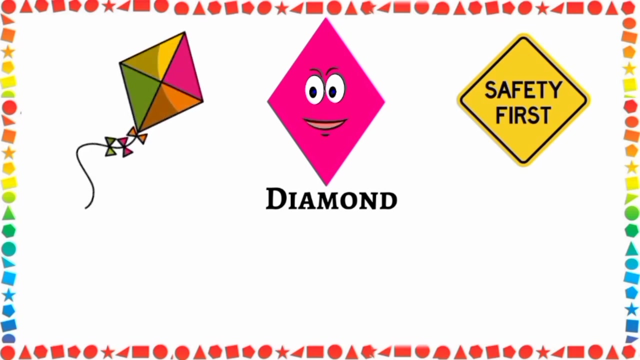 1,, 2,, 3 and 4. My 4 sides and 4 corners make me a diamond. You can find me in many objects around your surroundings. For example, You can see me as a signboard. You can fly me as a kite. 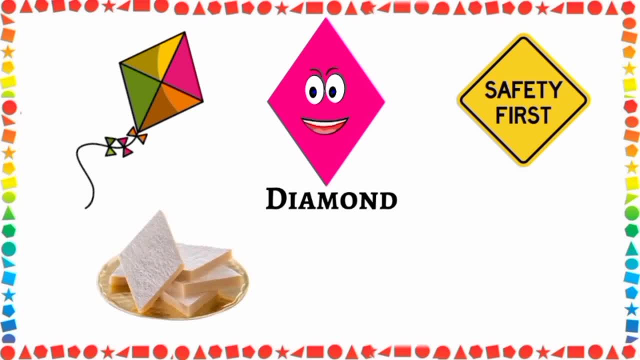 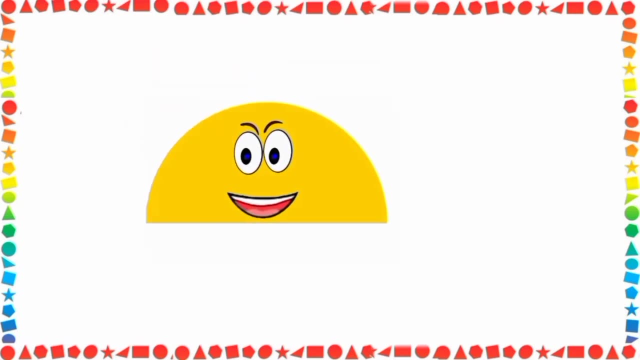 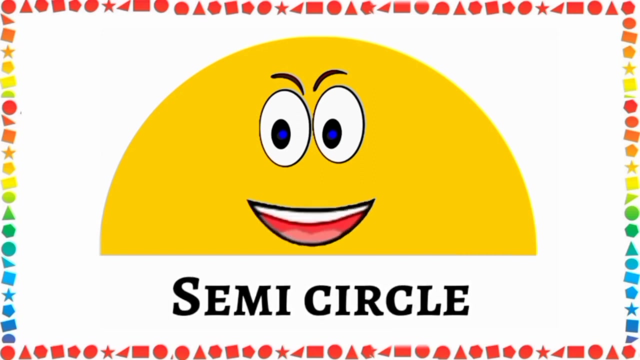 You can relish me as a sweet, You can wear me as a jewellery. All these objects can be seen in a shape of a diamond. Hi, I am a semicircle. I am half of a circle. I am made up of one curved line and one side. 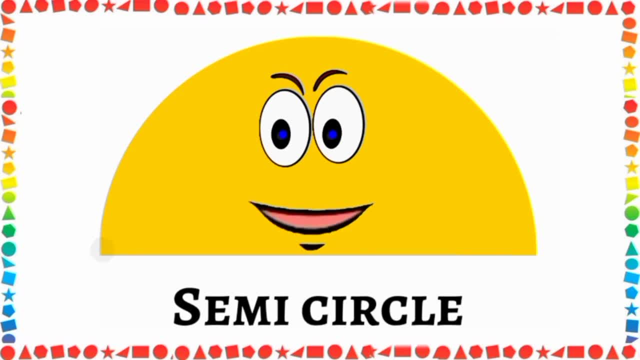 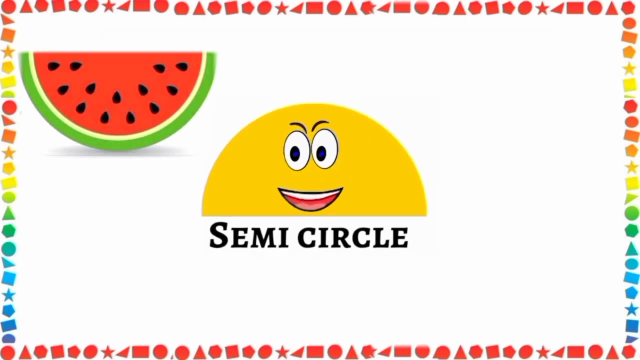 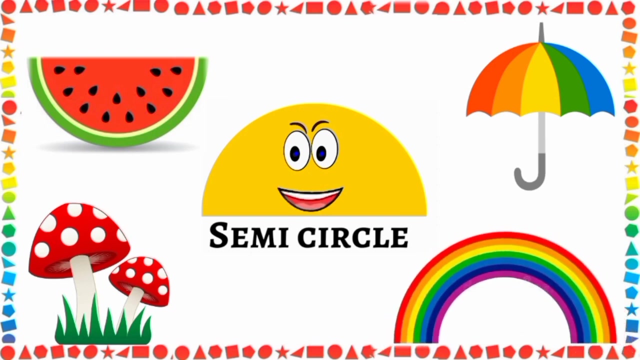 I have two corners, 1 and 2. You can find me in many things around you. For example, You can eat me as a watermelon slice, You can use me as an umbrella, You can water me as a mushroom plant And you can view me as a rainbow. 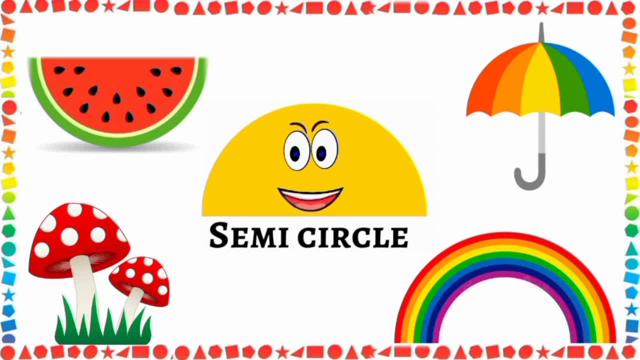 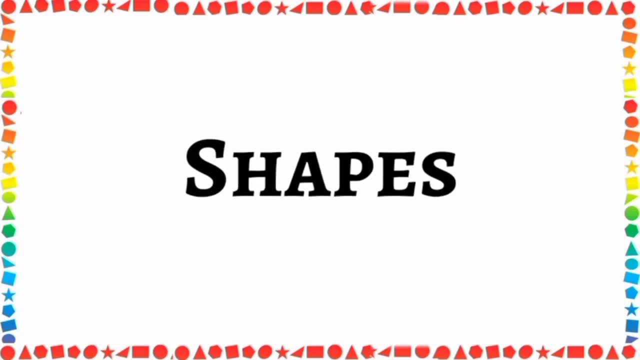 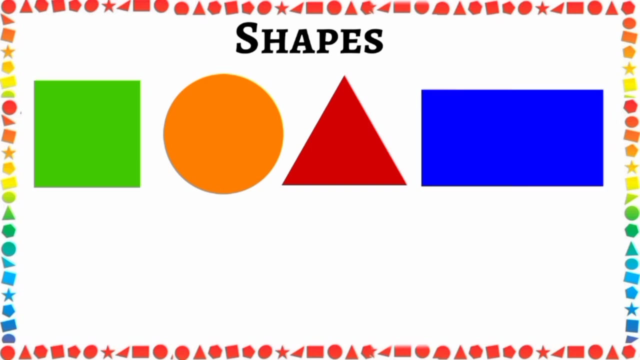 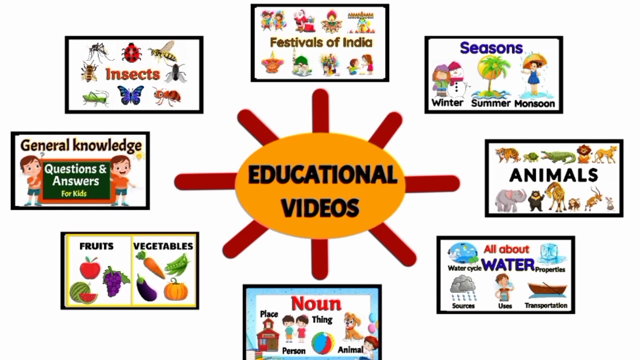 All these things can be seen in a shape of a semicircle. Now let's quickly revise the shapes we've learnt: Square, Circle, Triangle, Rectangle, Star Circle, Diamond, Semicircle And oval. For more educational videos, please find the links given in the description box. 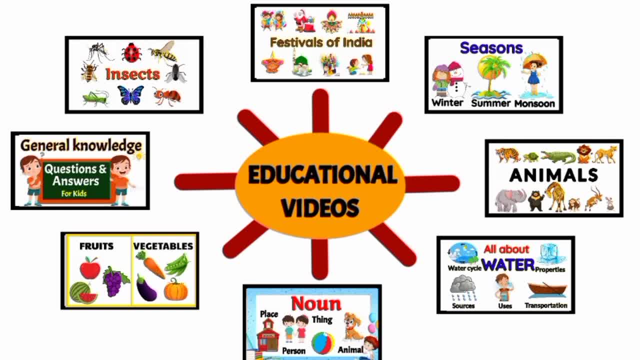 Thank you for watching. Do subscribe to our channel.